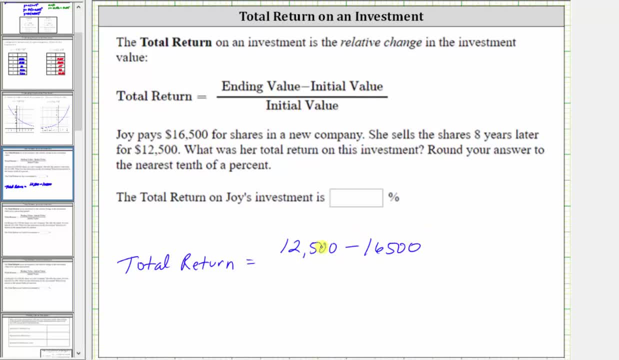 of $16,500. And this is divided by the initial value, which again is $16,500.. Well, 12,500 minus 16,500 is negative 4,000.. So we have negative 4,000 divided by 16,500.. 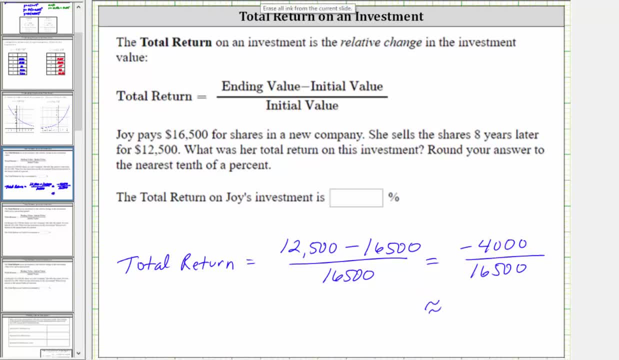 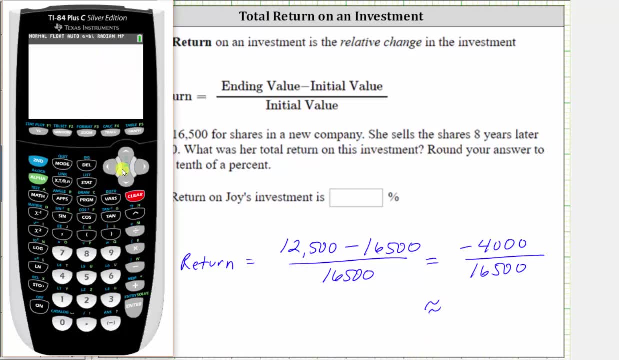 And now we need to find this quotient Because we're told to run a decimal to the tenths place value or one decimal place. we'll have to round the decimal to three decimal places. We have negative 4,000 divided by 16,500.. 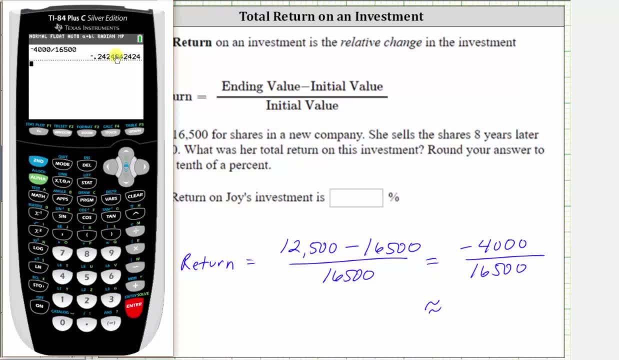 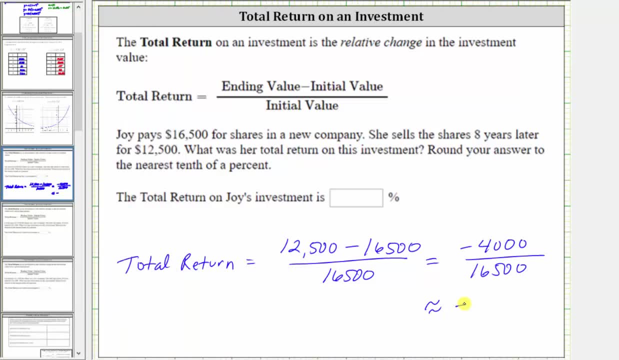 So notice how there's a four in the fourth decimal place, which means to three decimal places. this is approximately negative 0.242.. We had to round this to three decimal places. so we'll have to round this to zero is because, when converting to a percentage, 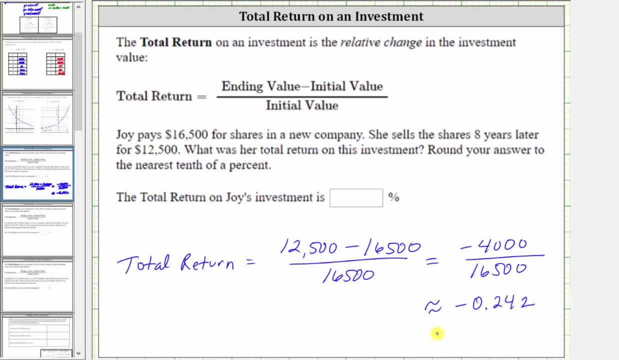 we will then have one decimal place, So as a percentage, we would have negative 24.2%. It's negative because she experienced a loss in this investment. Notice how she bought the shares for $16,500, and then she sold them eight years later for $12,500,. 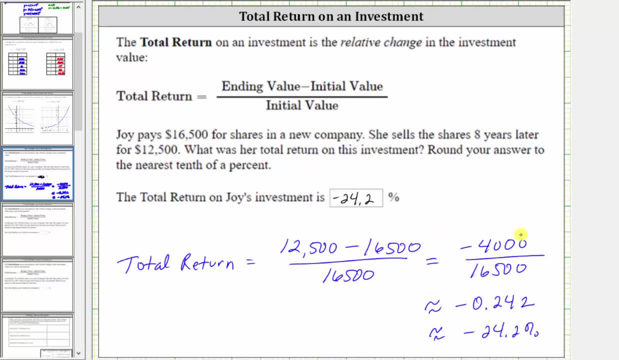 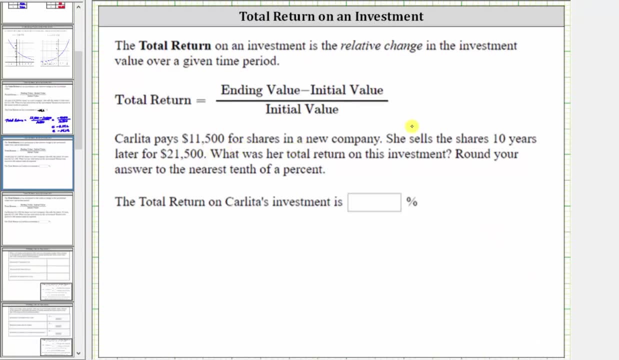 which is a loss of $4,000, which shows here in the numerator. Let's take a look at a second example. Carlita pays $11,500 for shares in a new company. She sells her shares 10 years later for $21,500. 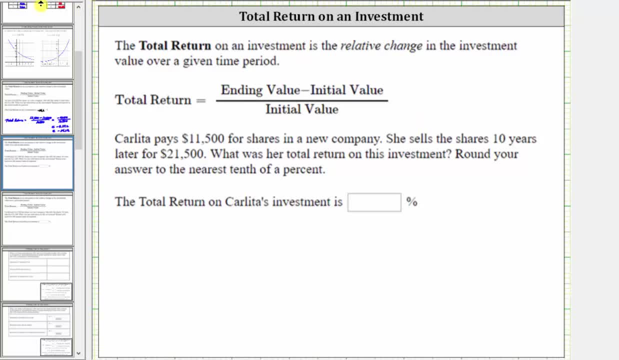 What was her total return on this investment? So again, the total return is equal to this quotient here, where in the numerator we have the ending value minus the initial value. The ending value was the sell price 10 years later of $21,500.. 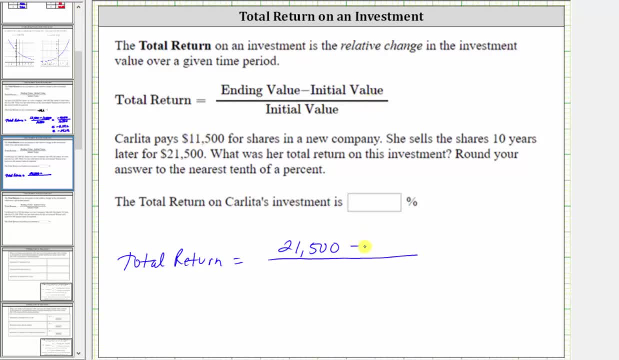 Minus the initial value, which was the purchase price of $11,500.. And then we divide this difference by the initial value, which again was the purchase price of $11,500.. 21,500 minus 11,500 is 10,000..